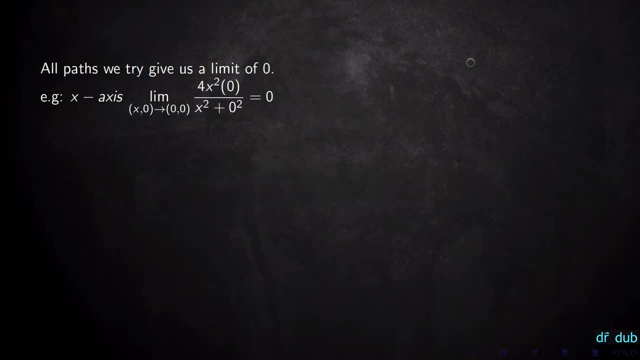 going to start with a function f of x- y and we're going to start with a function f of x- y, and we're going to start off by saying: okay, well, what we typically do is we apply the approach where we try to disprove the limit exists by taking different paths to the point, And this 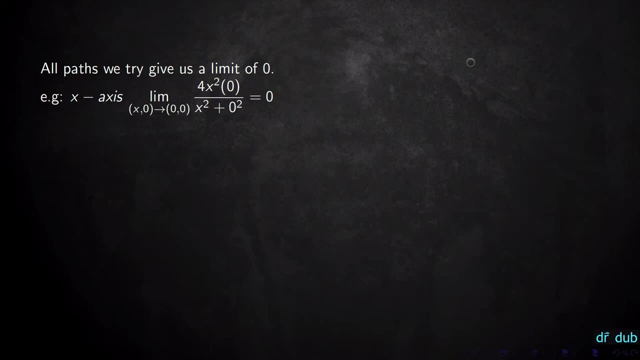 limit that we had is going to the origin. So we're going to take a path to the origin, the x-axis. that's the first path to the origin that we should try. That's: y equals zero. So if I plug in y, 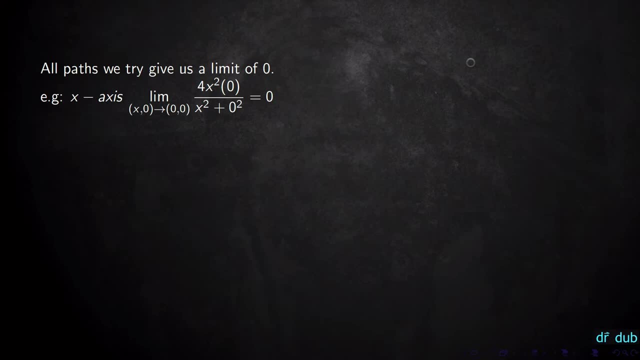 equals zero. then I get a limit of zero And so I try another one, maybe the y-axis, And I plug in x equals zero, That's the y-axis, And I get a limit of zero again And I say okay. 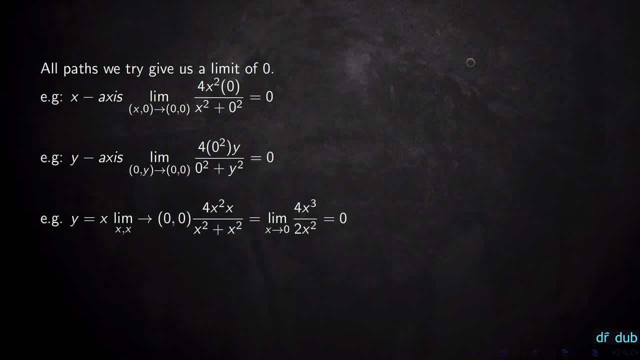 well, maybe I try another path that goes to the origin. maybe the line y equals x, So all of these paths go to the origin. So this is the limit as x, x goes to zero And this is going to be basically reduced down to 4x over 2, which is just zero again. So this is kind of 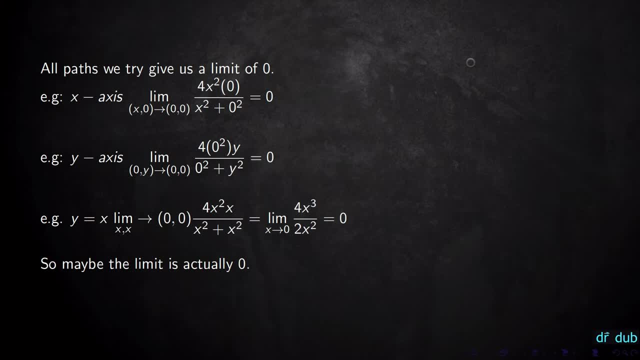 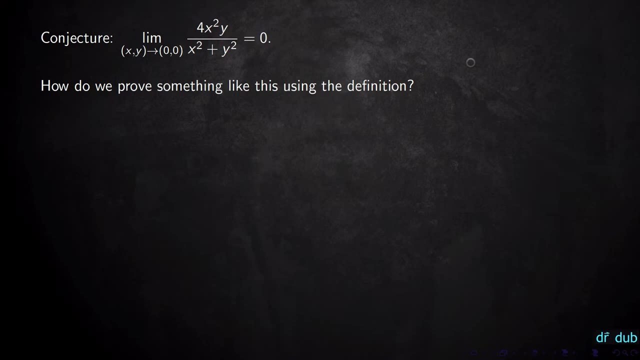 suggesting, maybe, that the limit is zero. So how do we actually show that the limit is zero? We have an idea of why it might be zero. Well, let's conjecture that the limit is zero. So how do we prove something like this using the definition? Well, we basically need to show that the definition 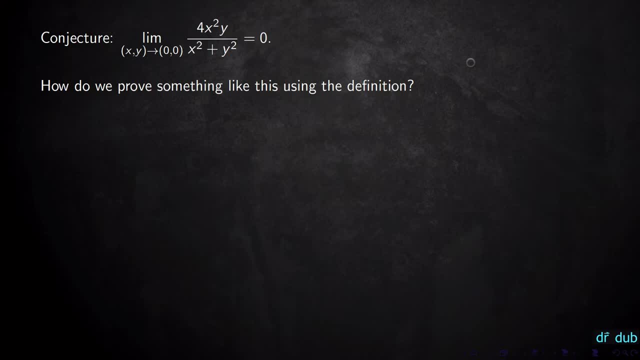 of this applies to this limit and this function, which means we need to show this inequality. is delta that we have to choose to get the distance from x, y to zero, zero, less than delta. We're going to choose a specific delta, So we're going to start off with this inequality right here and 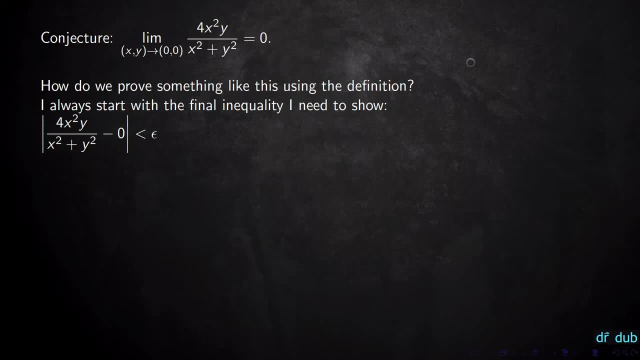 try to analyze it a little bit and maybe do some things with it that will help us. So probably what we want to do first is: what do we have to work with? What are we working with? Well, we're definitely going to have that the distance from x? y to the origin is less than delta. 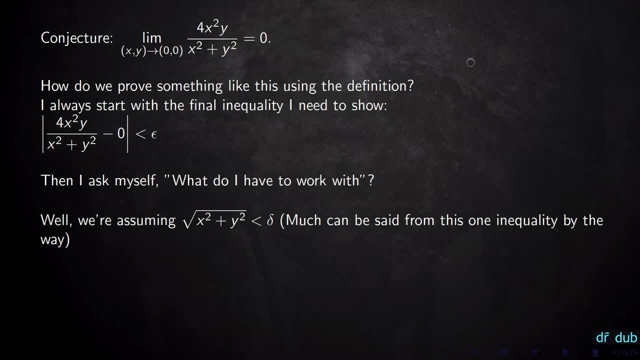 Which, if we rewrite that as x minus zero squared, that's just x squared, and y minus zero squared, that's just y squared. A lot can actually be said from this one inequality. For example, we could say the absolute value of x would be less than delta. We could say the absolute value of y would. 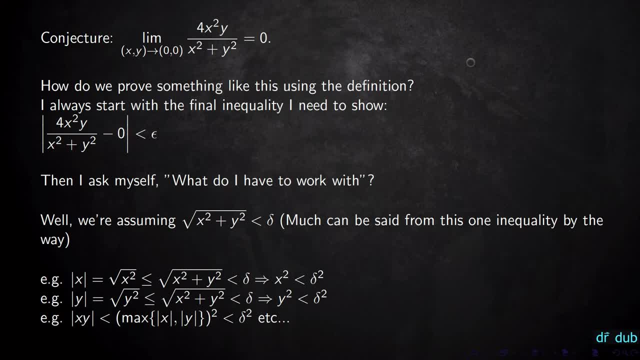 be less than delta, and the absolute value of xy would be less than delta squared. So there's quite a bit that we can say from just this one inequality that we're going to assume. So these are things that we will know for sure will be true once we set x squared plus y squared, the square root of that less than 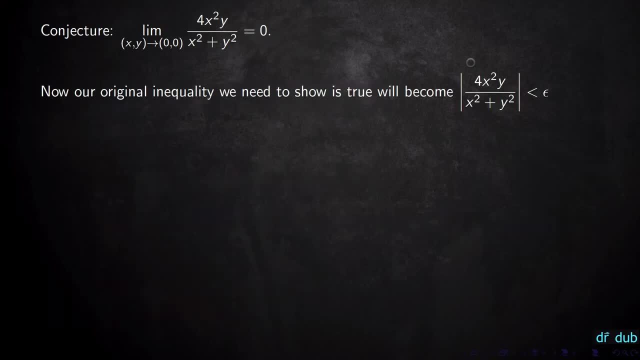 delta, All right. so now we're going to look back at our inequality and we say, okay, 4x squared y over x squared plus y squared minus zero, that's really just 4x squared y over x squared plus y squared absolute value. That's what we want to show, as less than epsilon. 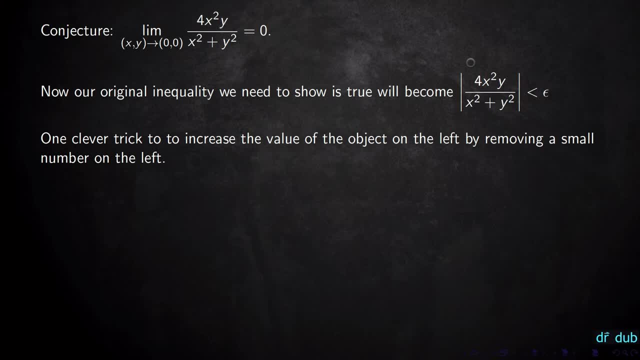 All right. one clever trick that we use to increase the value of an object on the left would be by removing a smaller number on the left. What we're talking about is the ratio x squared over, x squared plus y squared. If I get rid of that ratio, then the thing inside the absolute 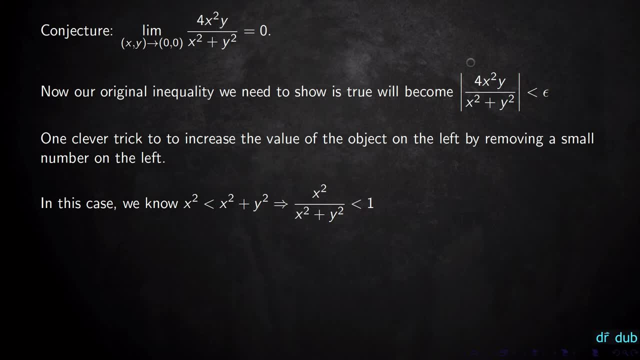 value will only get larger. So 4x squared, y over x squared, plus y squared, would be less than or equal to 4 times y inside that absolute value. So that is one trick. So that is one trick we can use to increase the value of what's on the inside of that absolute value. 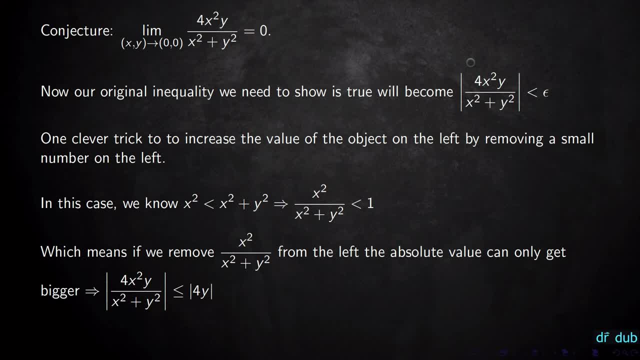 So if we remove x squared plus y squared, or sorry, x squared over x squared plus y squared, from the left, we can only get bigger. So basically, this inequality is definitely going to be true, for sure. You might say: how do I know? x squared is less than or equal to x squared plus y squared. 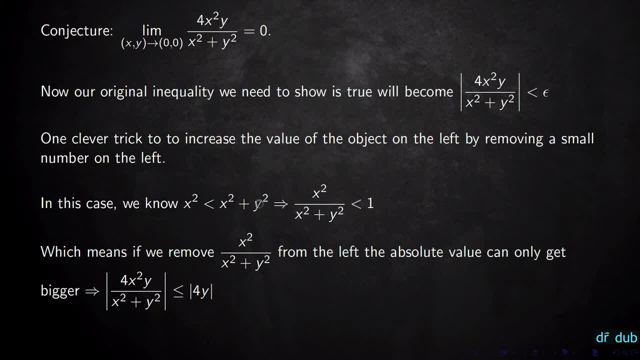 Well, these are real numbers. y squared is at least zero, So x squared is definitely less than or equal to x squared plus y squared should be equal to. right there, Less than or equal to. And same thing here: less than or equal to. 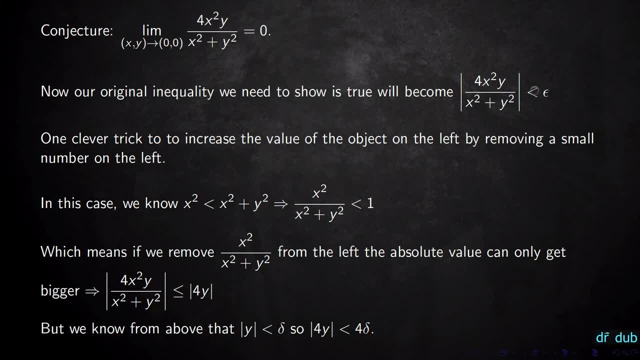 All right. so from above we know that absolute value of y was less than delta, So absolute value of 4y would be less than 4 delta. So this is starting to indicate what we should choose for delta If we want this thing to be less than epsilon.